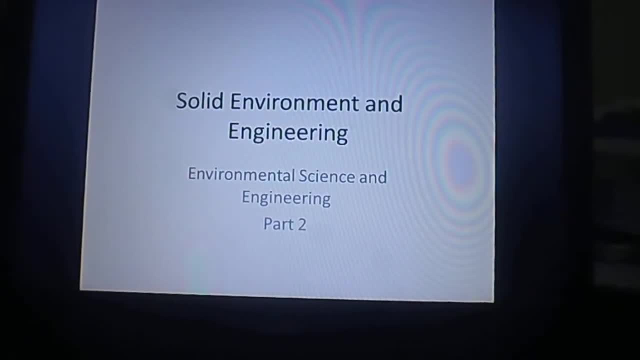 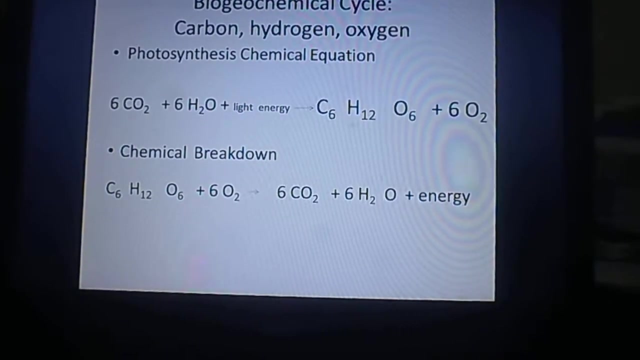 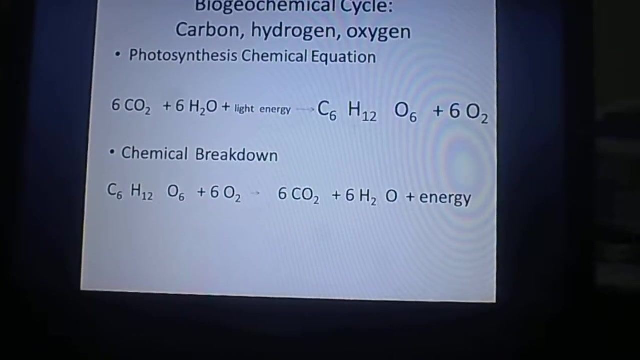 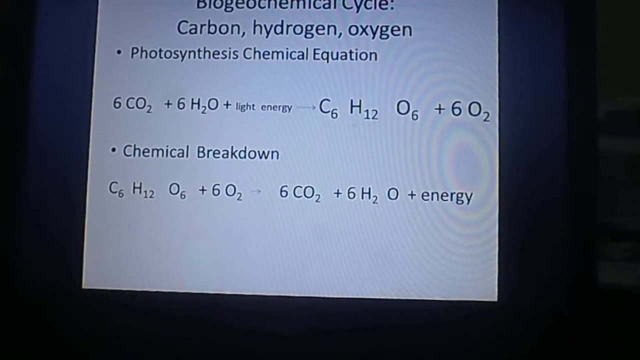 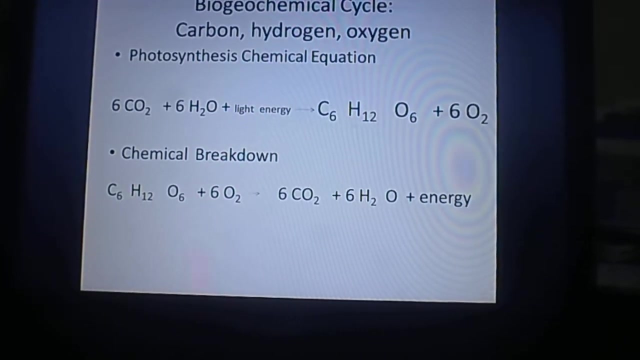 This is a continuation of the lesson on solid environment and engineering in the environmental science and engineering. subject: Carbon hydrogen and oxygen are elements which are cycling in the biosphere. Each of these may be involved in a particular biogeochemical cycle. Shown is a. 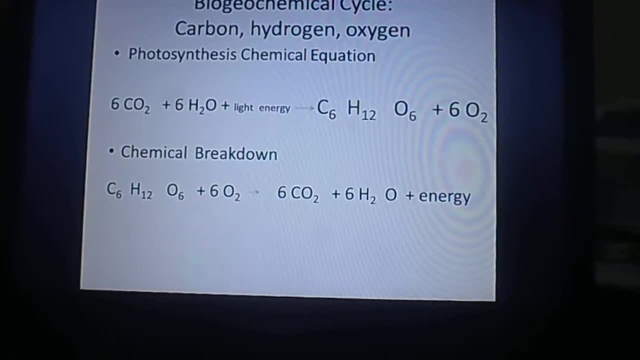 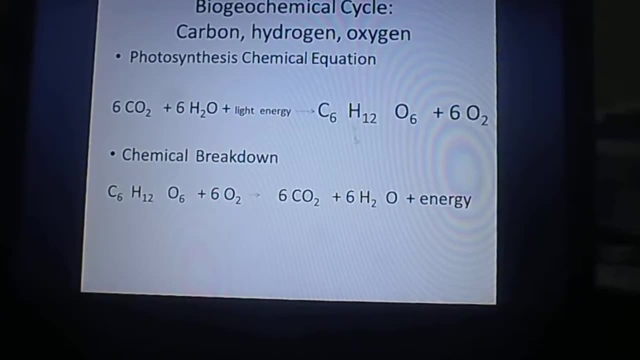 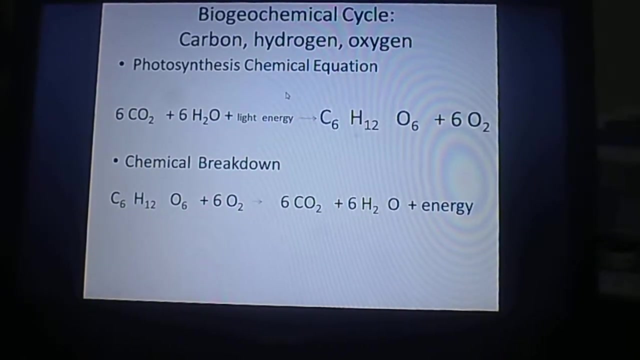 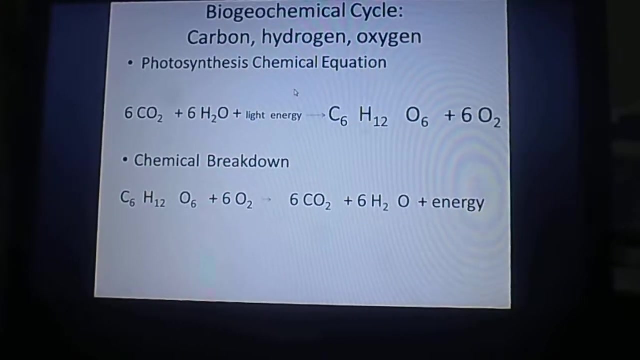 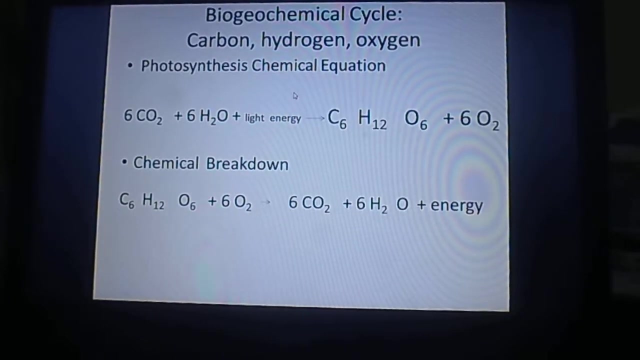 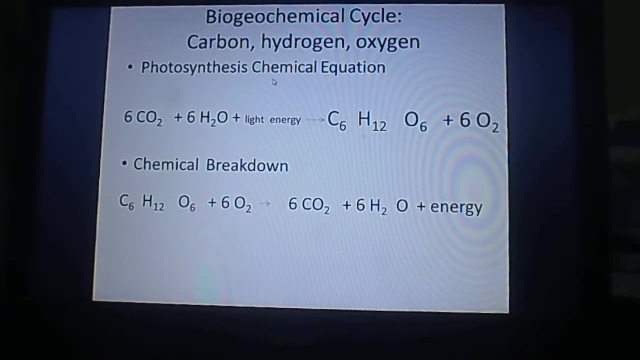 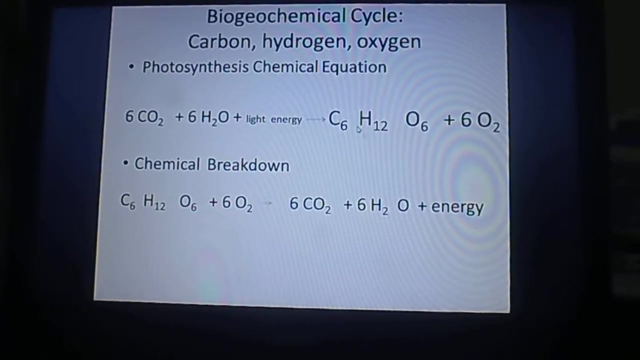 photosynthesis chemical equation showing carbon, hydrogen and oxygen as elements involved in the process Procesings. photosynthesis can be involved in a particular biogeochemical cycle. For instance, it is involved in the carbon cycle. Notice how the carbon is. Brooklyn gas steal T CSS is coming out of that process. 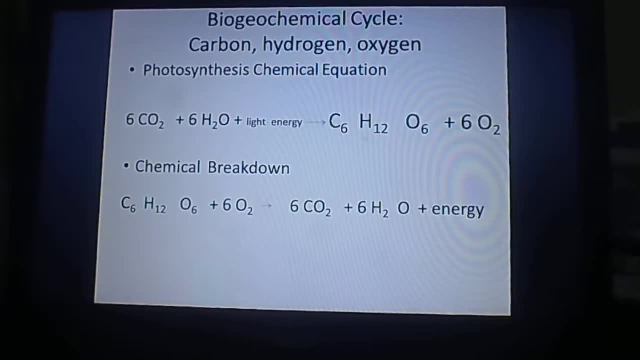 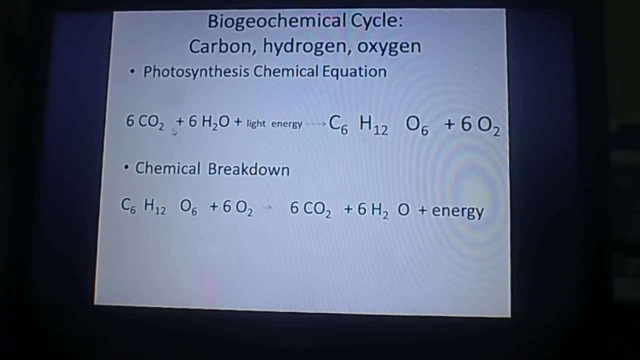 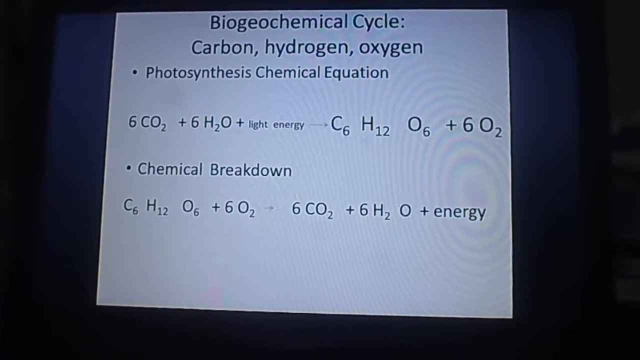 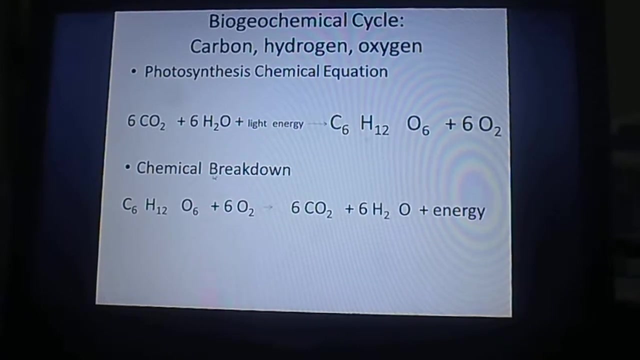 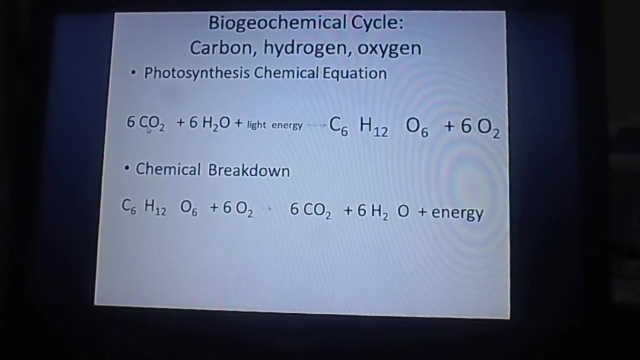 element is present in the carbon dioxide in the process of forming a type of carbohydrates in the presence of sunlight, during the photosynthesis process, when the carbohydrates will undergo chemical breakdown, carbon dioxide containing carbon is released. hence carbon is again cycled back, which can be used again during the photosynthesis. 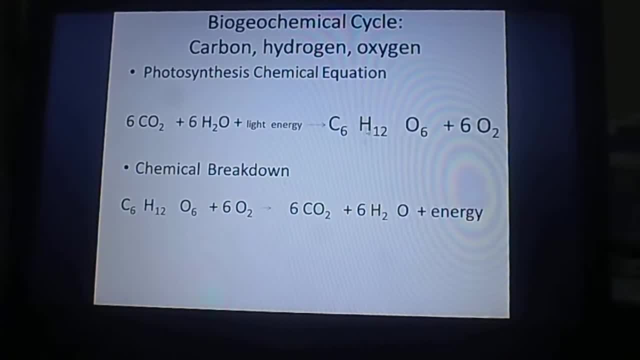 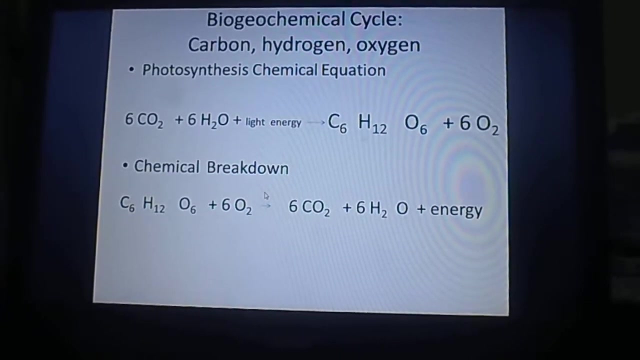 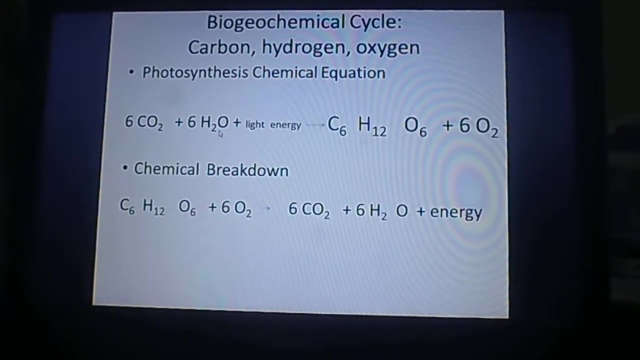 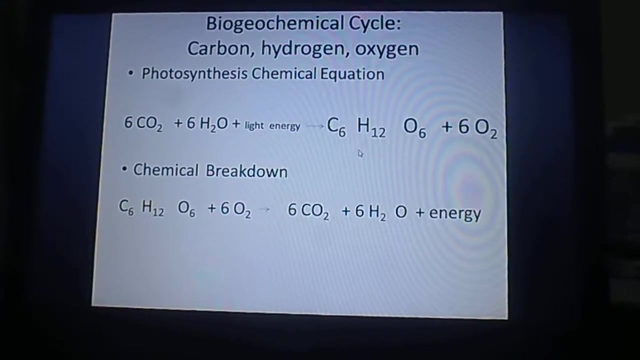 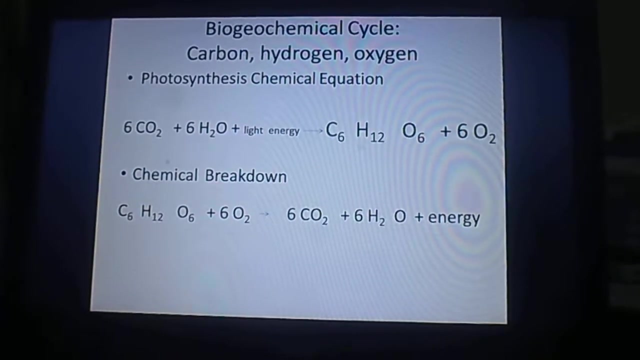 process to reduce the type of carbohydrates. so the cycling continues as carbon element cycles in the biosphere. notice how water is involved in the photosynthesis and hence hydrogen and oxygen elements involved in the photosynthesis process and therefore in the cycling. notice how hydrogen is also cycling from photosynthesis to chemical breakdown and back to the photosynthesis process. 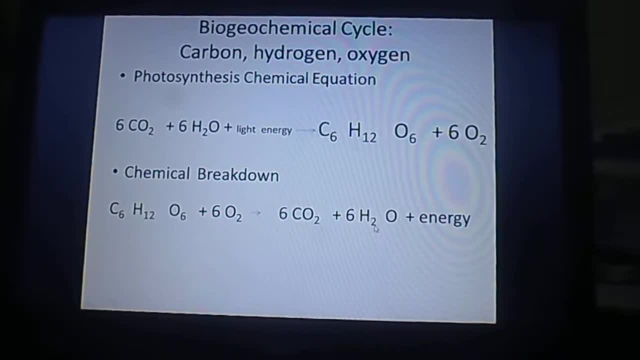 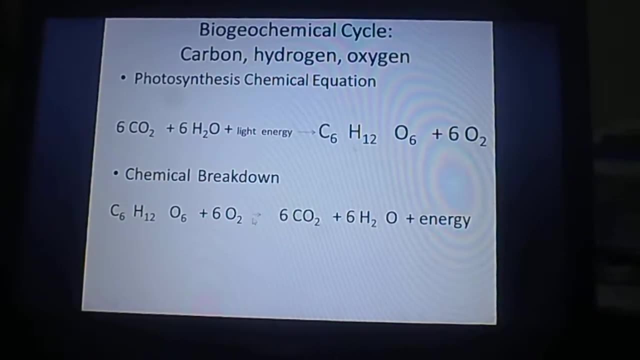 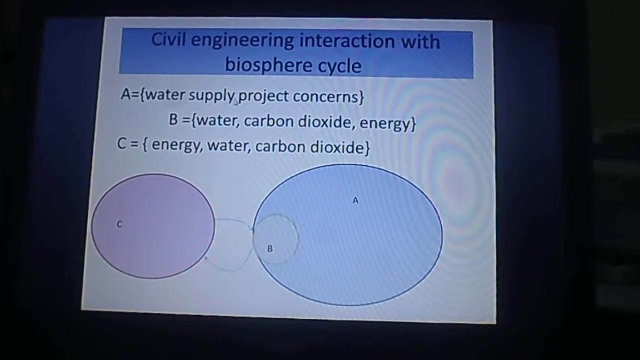 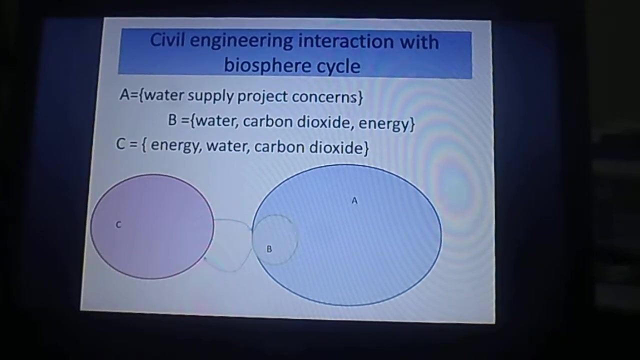 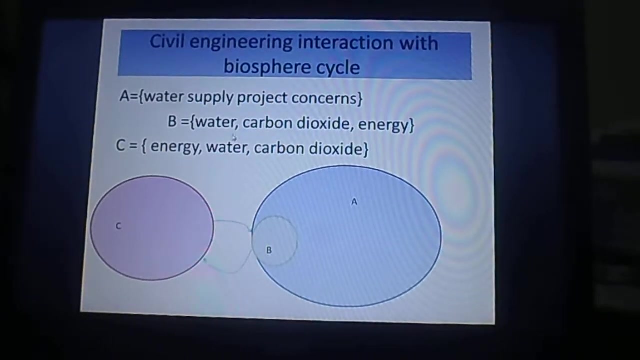 oxygen is also cycling from photosynthesis to chemical breakdown in a water supply project. the environmental concerns may cover water, carbon dioxide and energy in a water supply project. the environmental concerns may cover water, carbon dioxide and energy In a water supply project. the environmental concerns may cover water, carbon dioxide and energy. 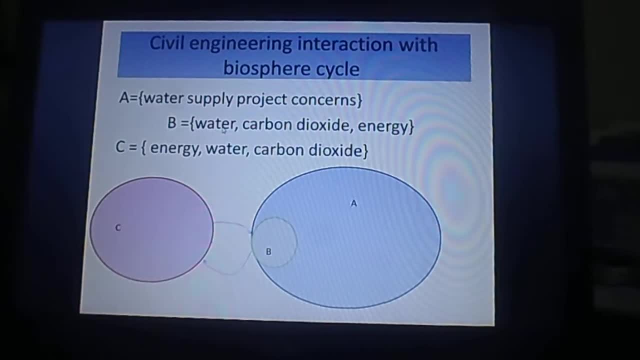 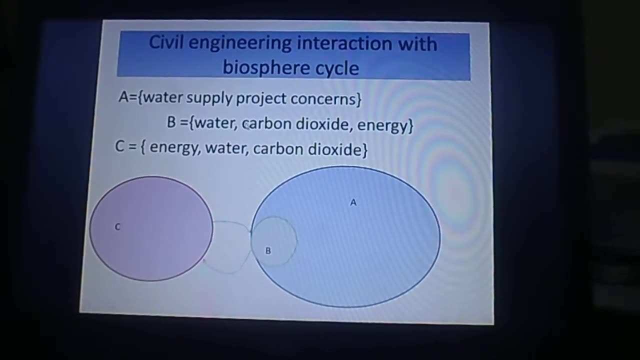 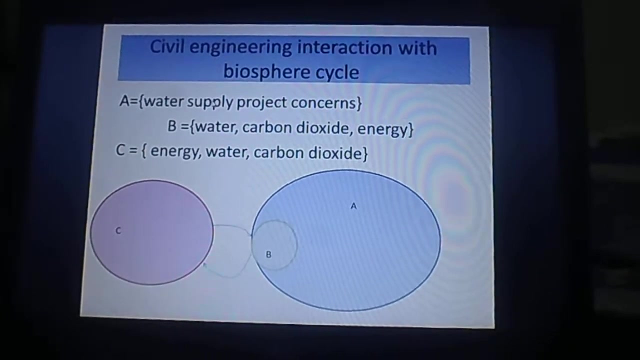 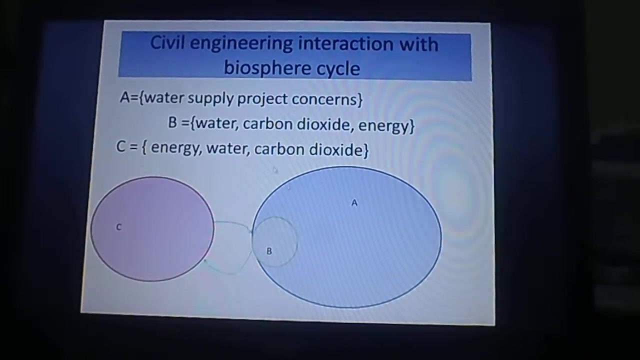 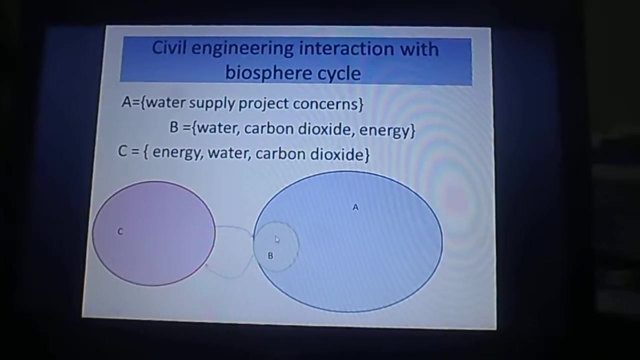 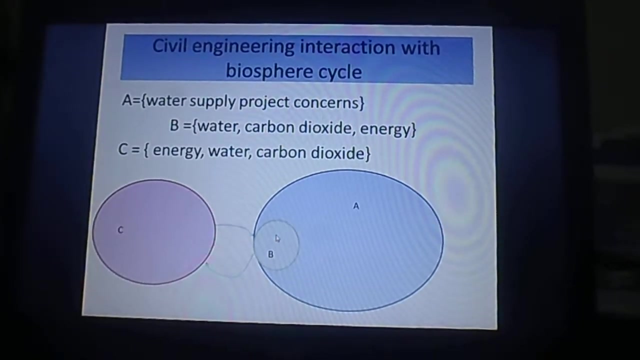 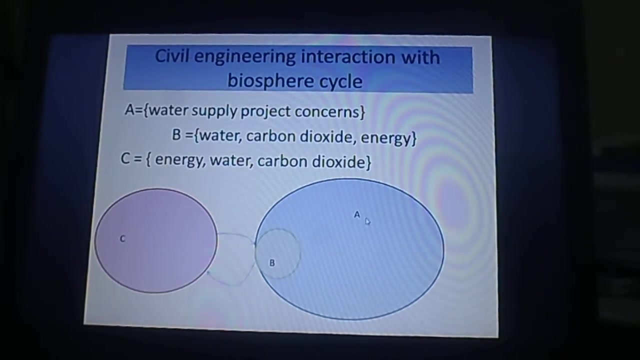 in the same, the same, in photosynthesis, the processes such as that. if these items are in the set of items misleading, which are environmental concerns of the water supply project, then which are environmental concerns of the water supply project? then set B, having these items as elements, is subset of set a, set a being the set.